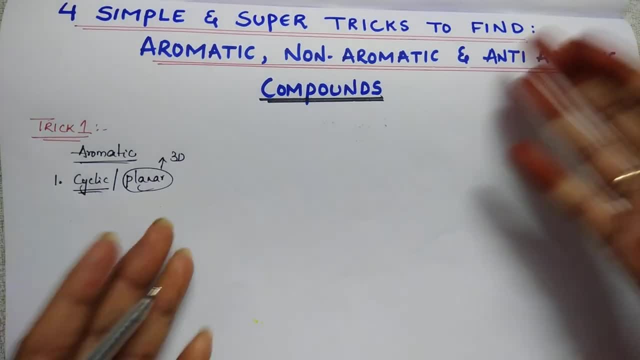 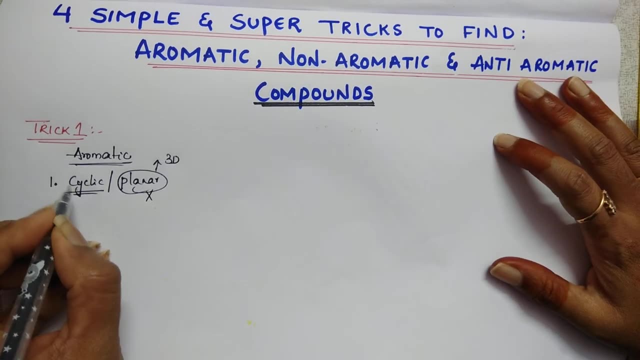 3D, point 3D view Every structure. what we draw on the paper, it is obviously a 2D, So we can't tell whether it is a planar or not by seeing. So if you find it is cyclic or not, it is enough. 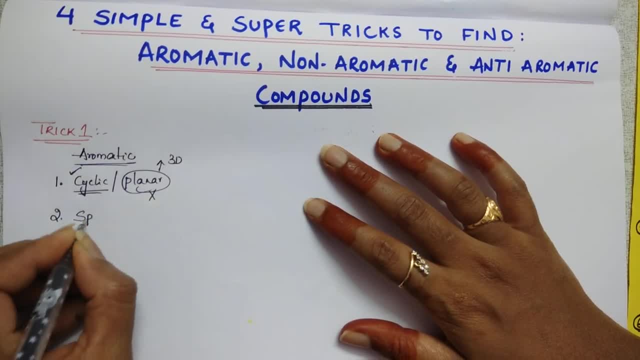 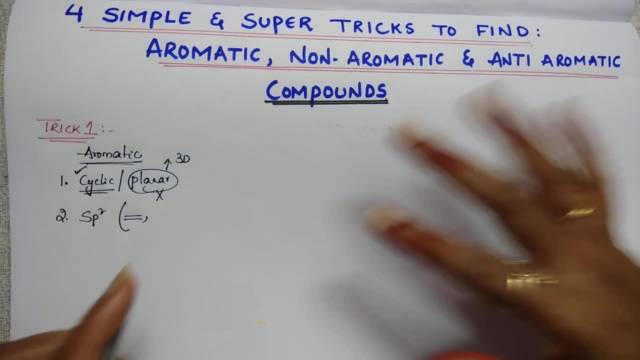 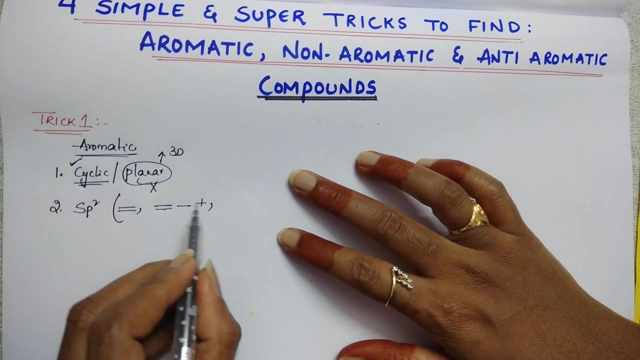 Point number two: every carbon should be sp2 hybridized, Like double bond should be connected to the carbon or any Other conditions like double bond should be in a conjugation with a positive charge. I mean double bond sigma positive charge should be there, or double bond sigma lone pair should be there, or 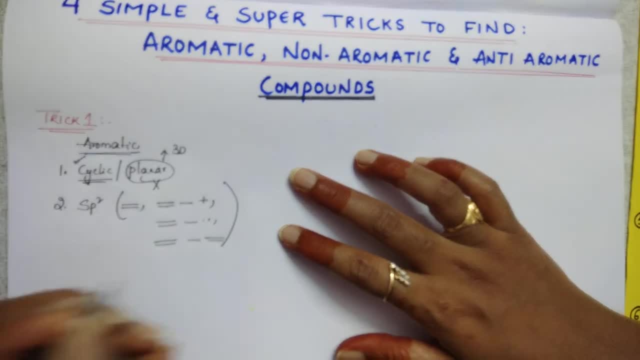 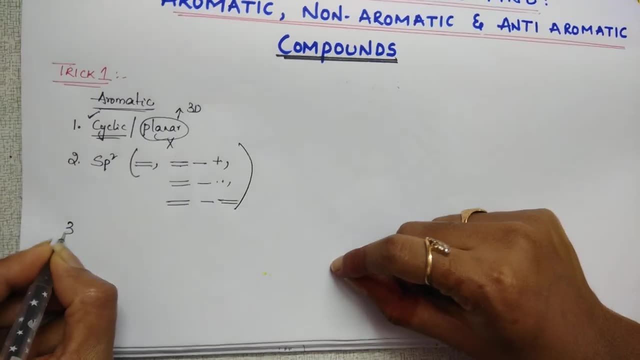 double bond, sigma pi double bond Like this. if it is there, we can say that carbon is sp2, hybridized carbon. This is another point. And the third one is: it should obey Huckel's rule. What is this Huckel's rule? It should obey Huckel's rule. It should obey Huckel's rule. It should obey Huckel's rule. 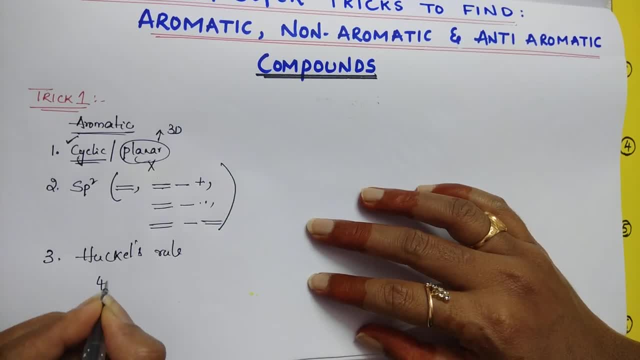 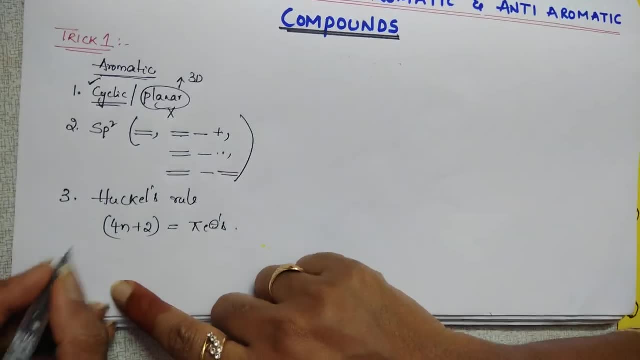 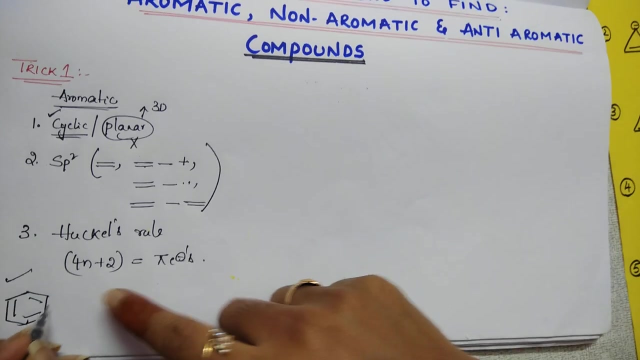 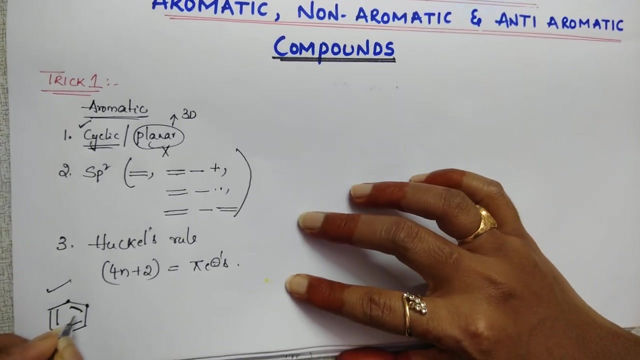 Again, we will see all the rules one more time. 4n plus 2 is equal to total number of pi electrons, total pi electrons. For example, let us see this benzene structure. Benzene is cyclic over Every carbon is sp2.. How to find? Because pi bond is there, so sp2.. Then, and total number of pi? electrons are 2.. One bond contains 2 electrons, So 2, and here 2.. And here 2.. Total: how many electrons are present? Total, 6 electrons are present. So 4n plus 2 is equal to 6.. Then 4n is equal to 6 minus 2. This comes 4.. n is equal to 1.. So 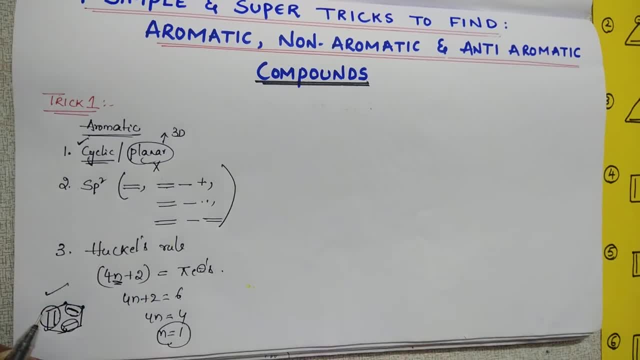 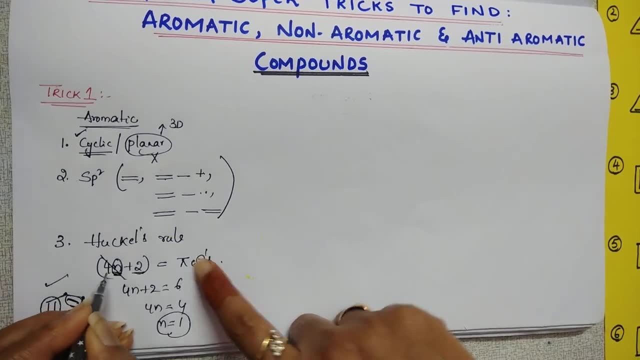 what I want to tell you is keep n. n is an integer. Keep n plus 0. If you put n plus 0, you get the total number of electrons 2.. If you get n plus 1, then 4 into 1,, 4 plus 2,. total 6.. Like that, keep different n values like 0,, 1,, 2,, 3.. You will be getting total number of electrons 2,, 6,, 10,, 14.. So what I want to tell you is, without doing any Huckel's rule, simply see cyclic sp2 are not, and either 2,, 6,, 10, 14 electrons is there, then it is aromatic Clear. Now the second one. If this is not the condition, let us see about anti-aromatic, Anti-aromatic, Anti-aromatic. Very easy, Cyclic first condition. 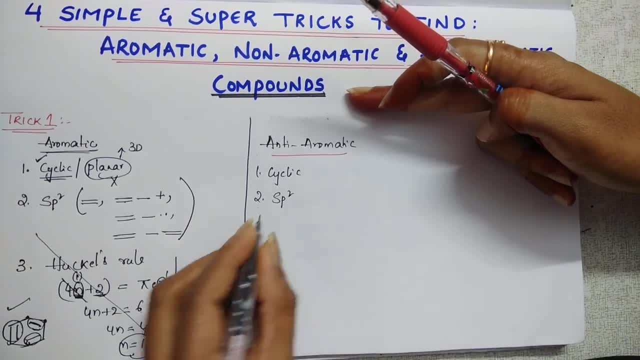 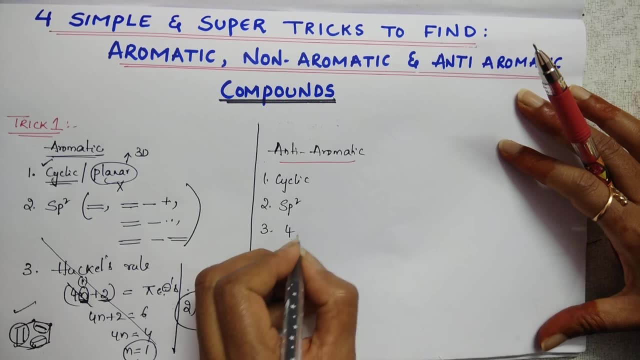 is same. Second is sp2 hybridization. Every carbon should be. And the third point is it should it should follow. it should not follow Huckel's rule. If it is having 4n, it is satisfying 4n, Like n plus 4n. If it is having 4n, it is satisfying 4n. If it is having 4n, it is. 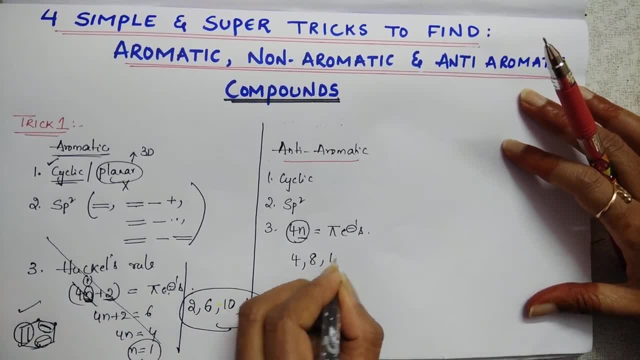 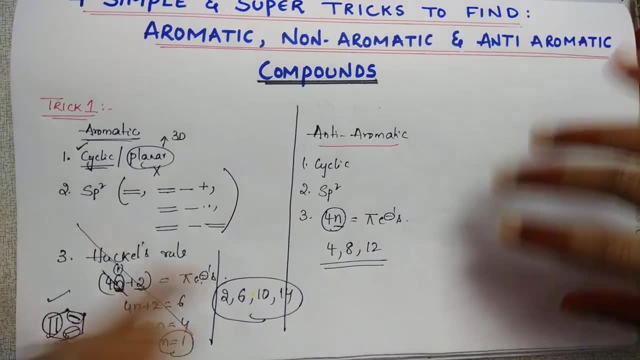 1,, then 4.. n plus put 2,, 8,, 12. If these electrons are there, then anti-aromatic Highly unstable. So if, if it follows it is, it is cyclic sp2 and it is following following. 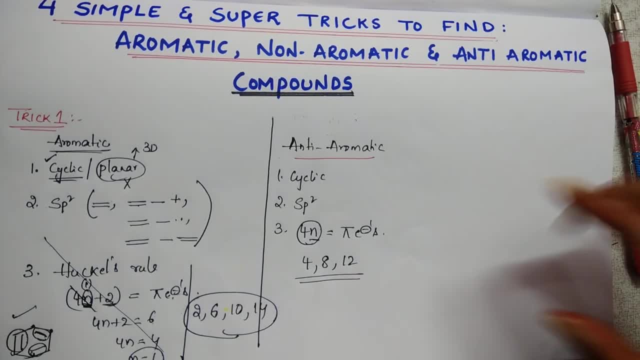 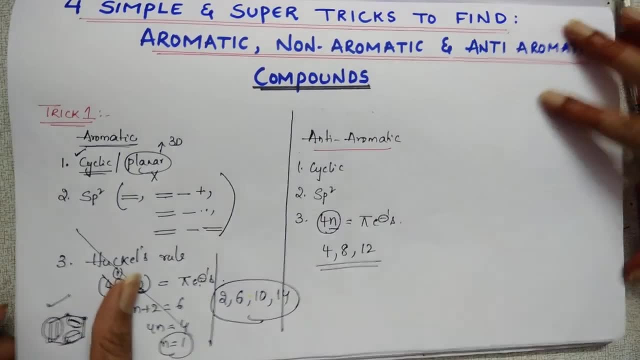 Huckel's rule, then it is aromatic. If it is not following that cyclic sp2, but not following Huckel, it is following that 4n plus 2, 4n rule, then it is anti-aromatic Now, if any. 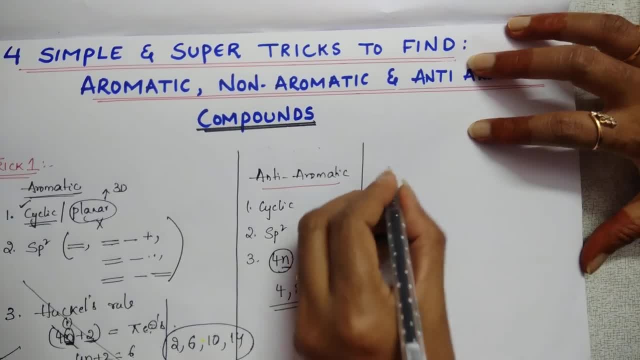 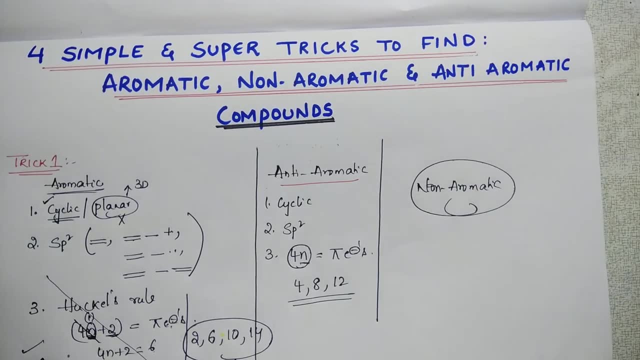 one of these conditions are there, then it is aromatic. If it is not following that 4n conditions it is not following, then it is non-aromatic. What is? the students tell me It is non-aromatic. When we say it is non-aromatic, can you say When it is not? 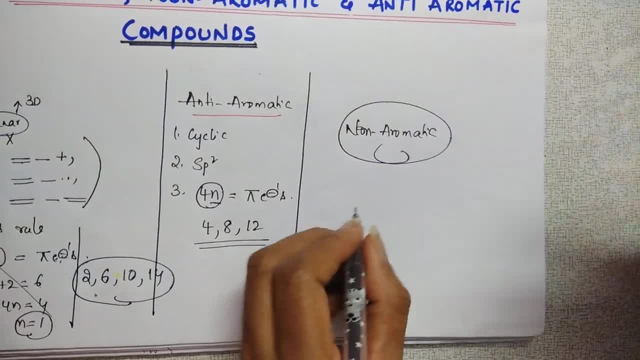 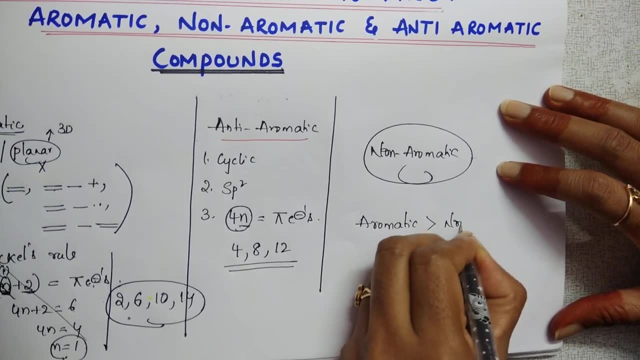 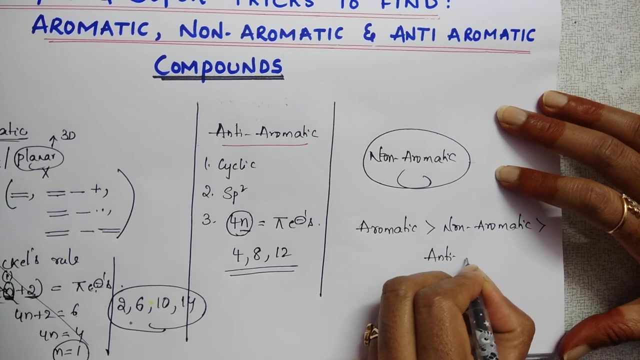 following any of any one of this rule. So, coming to the stability order, aromatic is more stable than non-aromatic, Then last is anti-aromatic. So in anti-aromatic, due to resonance itself, it is getting the instability We will see in another detailed session In. 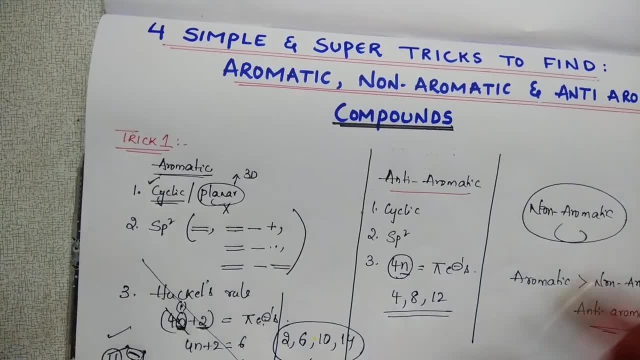 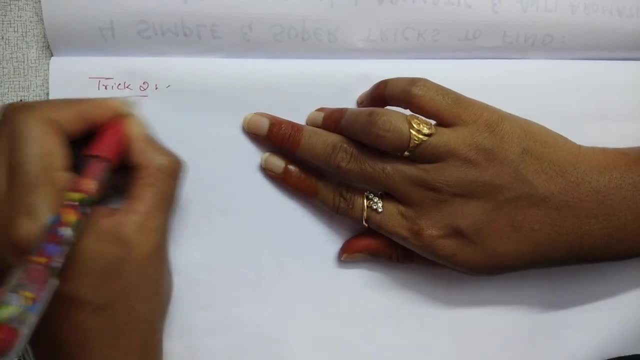 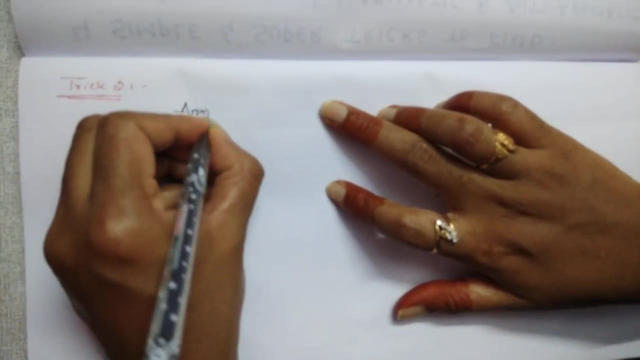 this class. I am going to teach you how to find it Trick. this is trick number 1. done, Trick number 1.. Now let us see the trick number 2.. In here I am going to teach you the main thing, that there are certain cases, Aromatic compounds. what you feel is when benzene 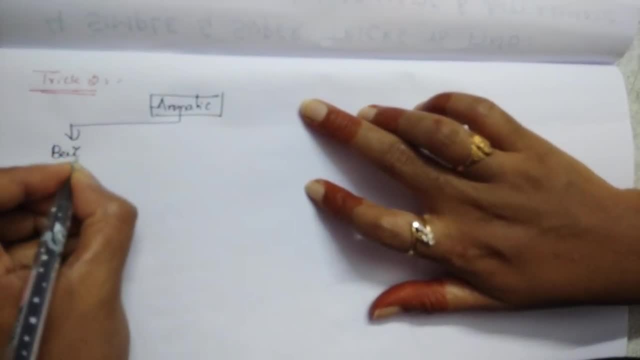 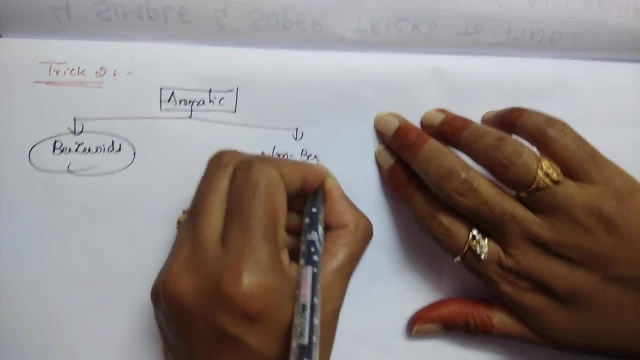 ring is there, only it is aromatic. But no, Compounds are of two types: One is benzenoids, another one is non-benzenoids. So if benzene ring is there, only if you think it is aromatic, then your answer is wrong answer. There are. 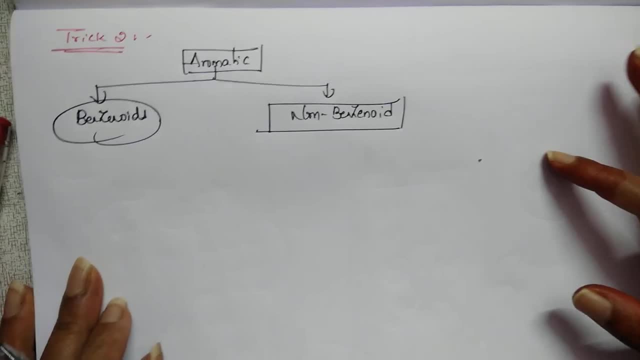 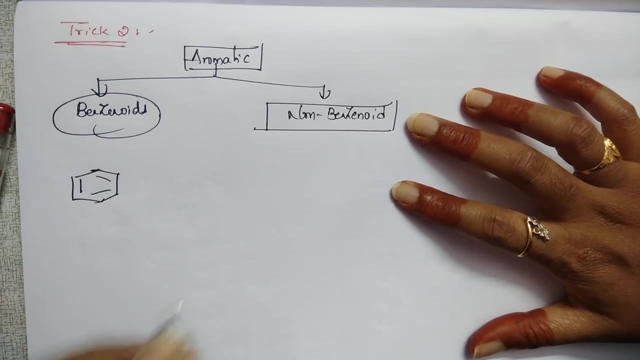 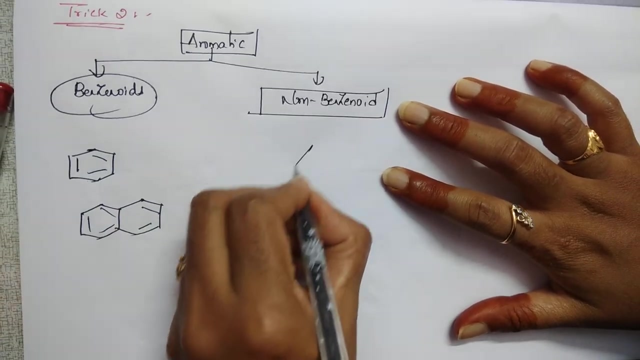 some compounds without benzene ring also. they are stable, They are aromatic. For example, benzene is there, It is having benzene ring, So you can say: aromatic Naphthalene, benzene ring is there. Okay, There are certain compounds without benzene ring also. they are aromatic, For example: 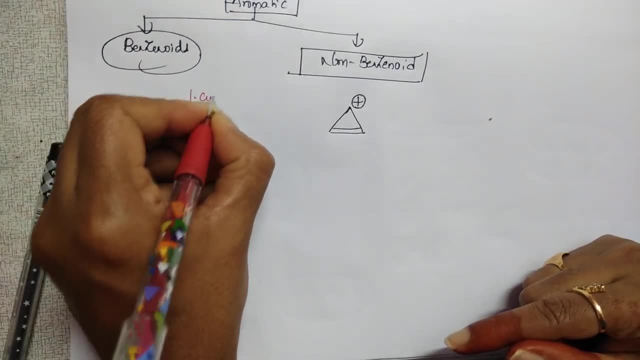 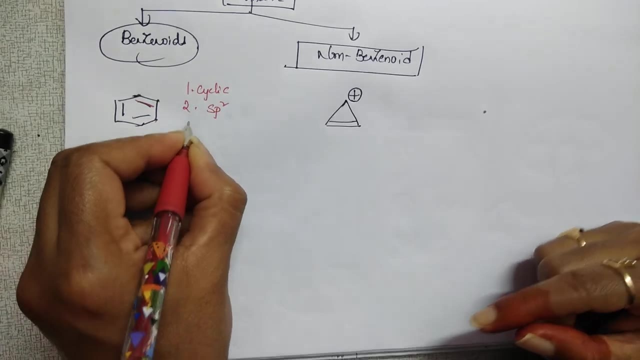 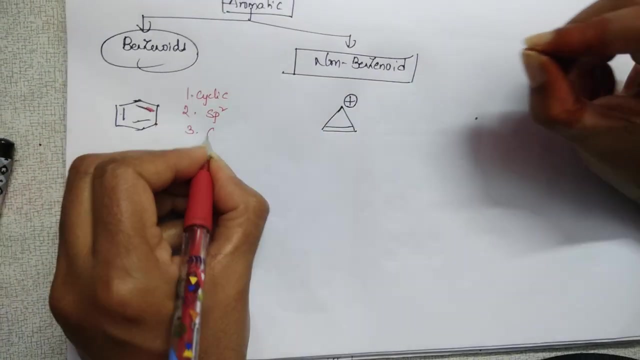 see in this case. One is, first point, cyclic. Second, every carbon is sp2.. Double bond is there, sp2.. Total number of pi electrons are: one bond contains 2 electrons, 2 plus 2 plus 2.. Total, 6 pi electrons. What I told you- 2, 6, 10 is there- means aromatic. 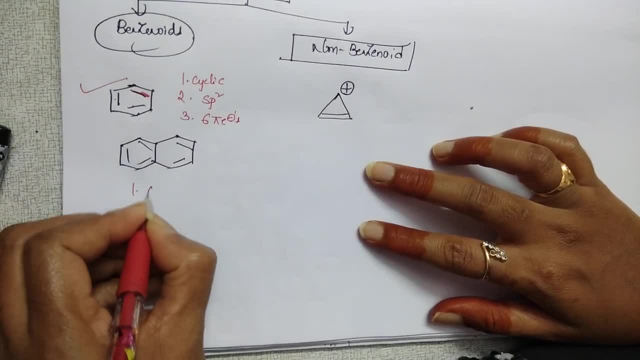 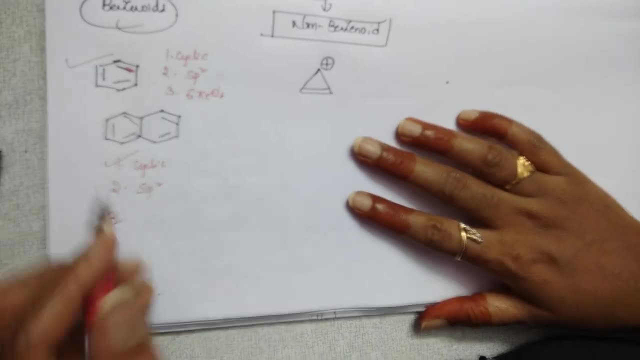 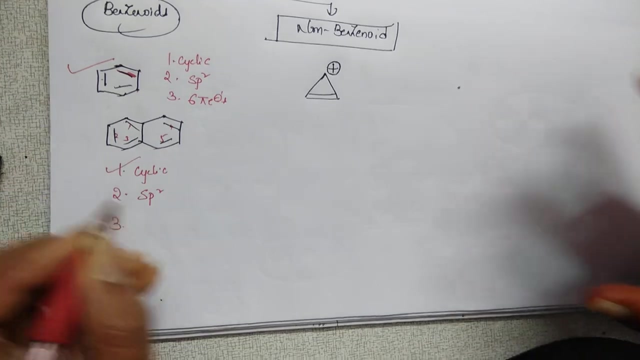 So this is aromatic, See here. First structure is: this is cyclic. First condition: satisfied Every carbon, have double bond, sp2.. Third one is here here total number of electrons you count: 1,, 2,, 3,, 4, 5 pi bonds are there. Each pi bond contains 2 electrons, 5, 2 are. 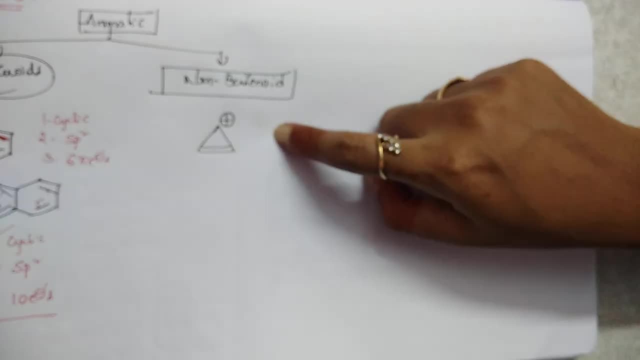 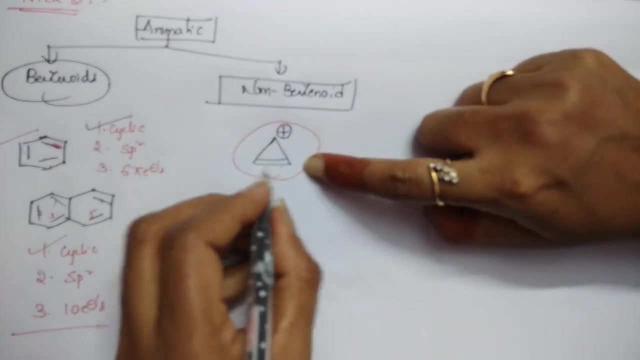 10 electrons, So aromatic. But see non-benzenoids. they are not having benzene ring, but they are aromatic. So count. it is cyclic, First condition satisfied, And see the second condition. It is cyclic, First condition satisfied. 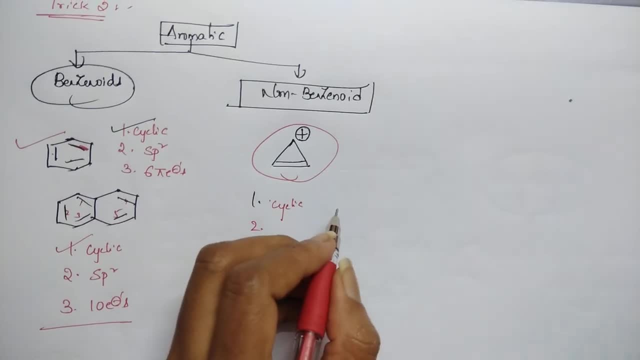 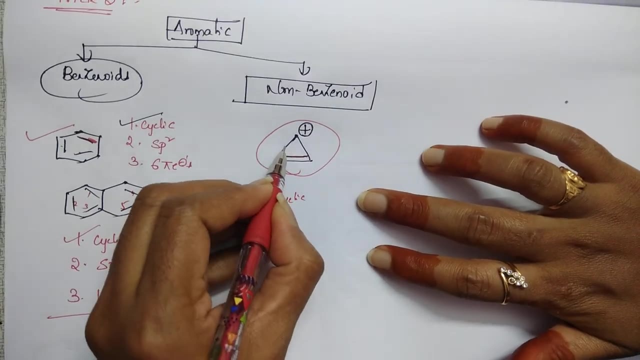 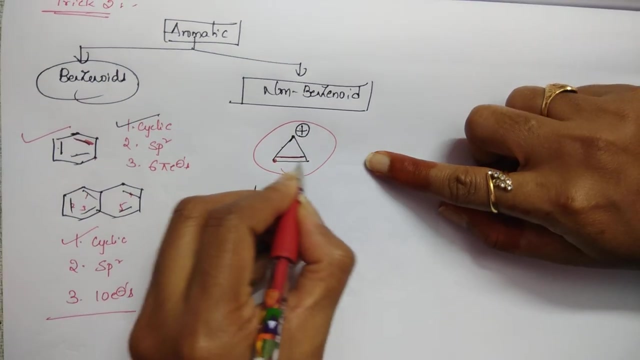 Second condition: you see sp2.. How to find sp2 or not Pi bond is there at this carbon. Okay, But this carbon, how to find? Simple technique, is pi sigma positive charge. It is one of the condition, Pi sigma positive. So this is pi sigma positive. This is also sp2.. Okay, 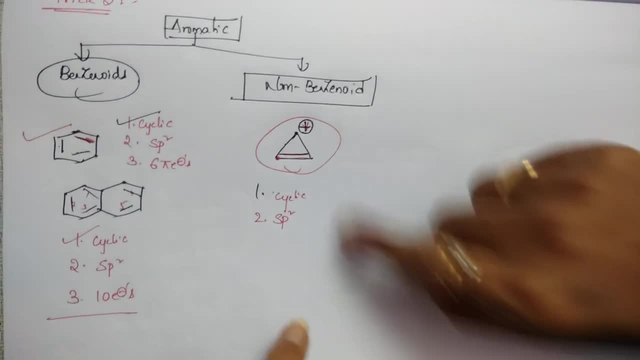 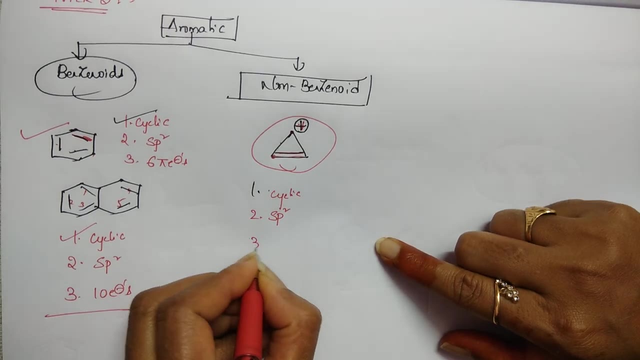 Reason I you know, you will come to know. This is a resonance, This shows a resonance. What is resonance? How it will exhibit. I already done the video. If anyone want to learn about resonance, you can watch that. And total number of pi electrons. how many students tell me here Only 2 pi electrons. 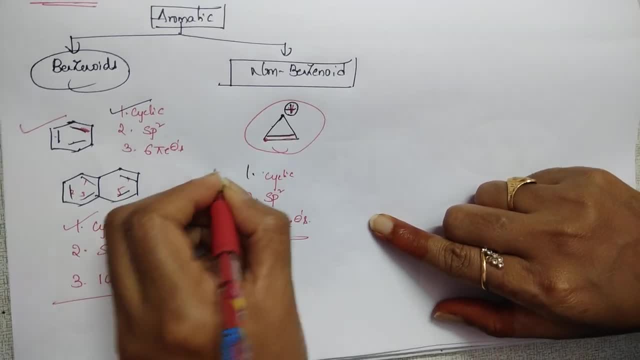 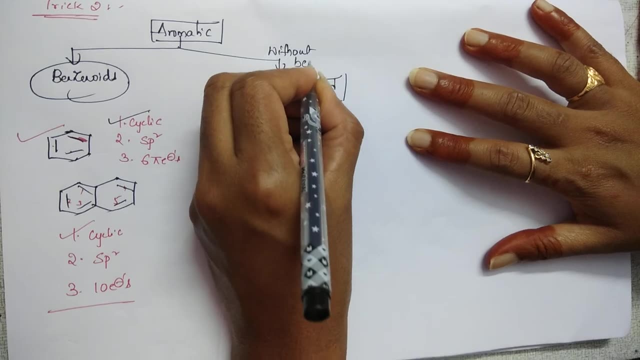 are there 2,, 6, 10.. What is that? Aromatic? So non-benzenoids means without benzene ring also they are aromatic. Without benzene also they are aromatic. This is important because if you see this kind of structure, you should not feel that it is not aromatic. So you 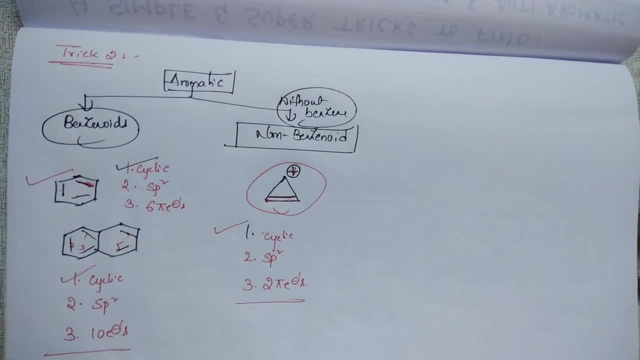 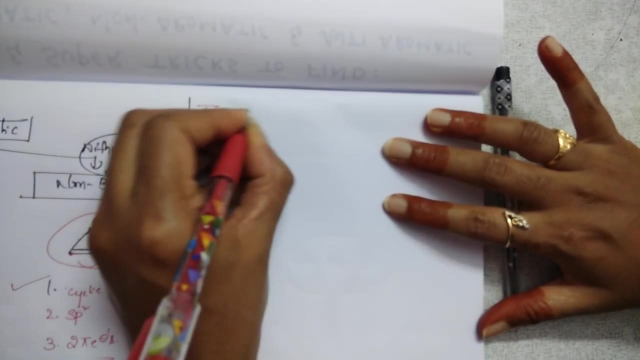 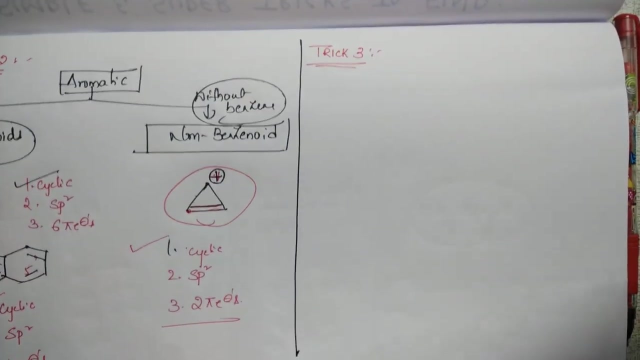 should not feel that it is not aromatic, Even though without benzene also, it is aromatic. Now let us see trick number 3.. Here I want to tell you that there are some compounds which are having a heteroatom. What do you mean by this heteroatom? Heteroatom means. 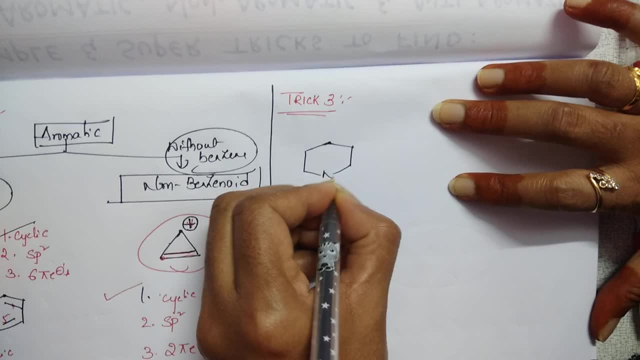 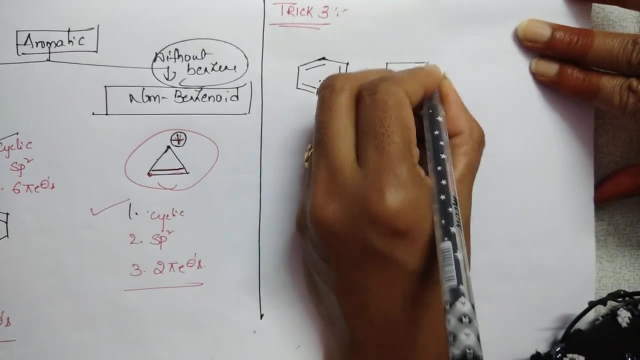 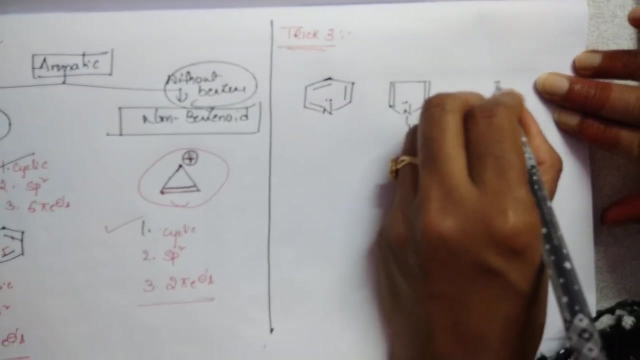 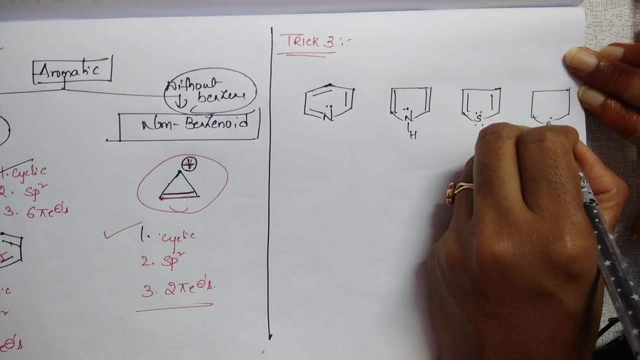 they have some different atom within the ring. For example, see here nitrogen, This is called pyridine, Pyridine, This is pyrrole, And you can see thiophene, furine like this. We have different structures. 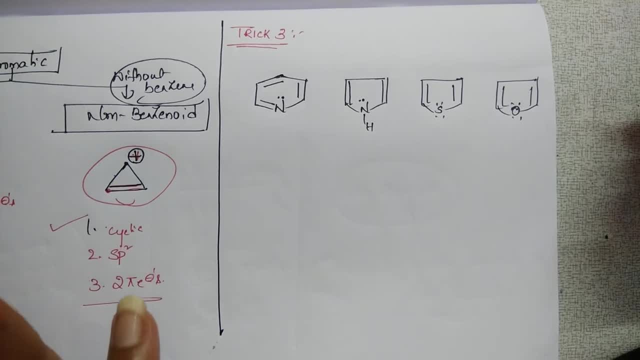 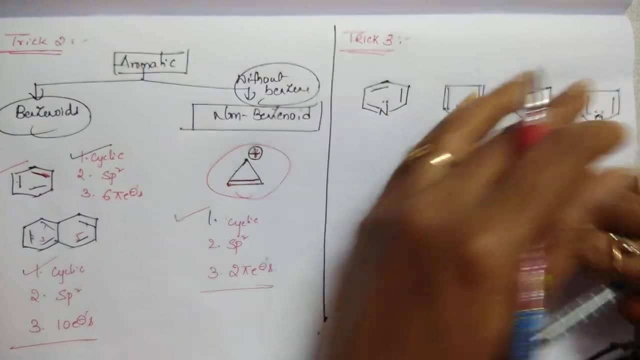 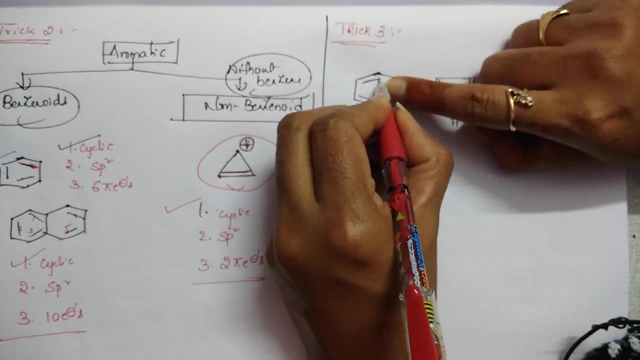 right, Whether it is, all these are aromatic. only How we will come to know whether these are aromatic or not. You can find that: see 2: cyclic, all are cyclic. every carbon is sp2, hybridized carbon, and here count the total number. 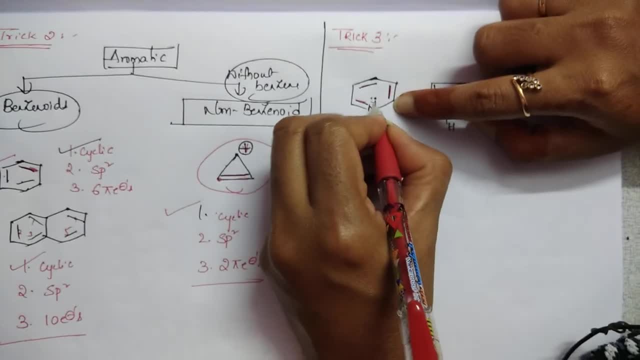 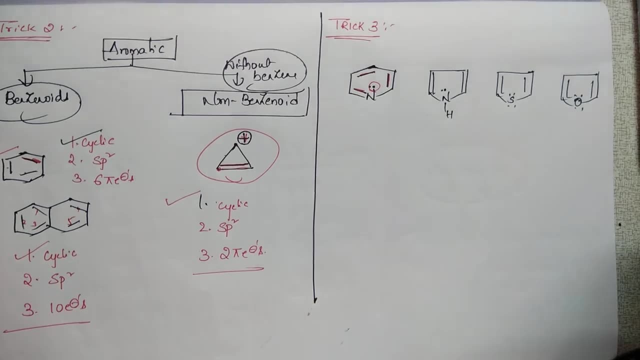 of electrons, 2 plus 2 plus 2, total 6, and if you count this 2 also, you will get 8, 8 means it is non anti-aromatic, right, but why it is aromatic? because this this: with this 6 electrons in the, 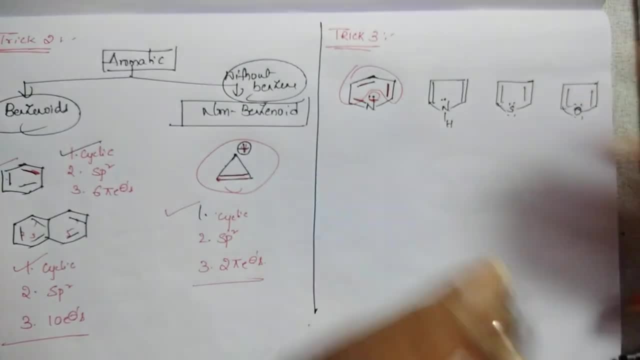 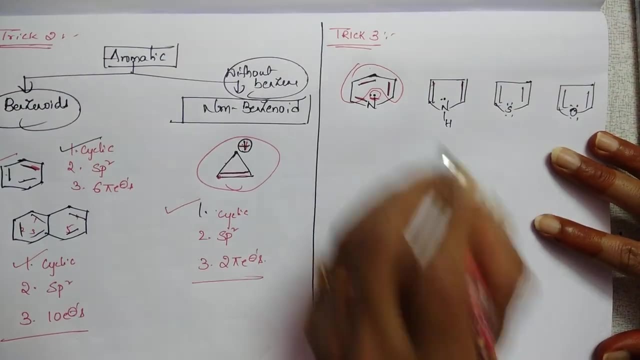 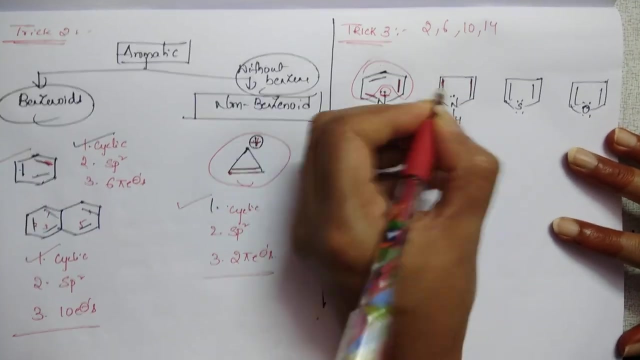 ring. it already got the stability. so the 2 electrons which are present in the nitrogen it don't involve in the resonance- see in this case 2 plus 2, 4 only to show the aromaticity should be 2, 6 or 10 or 14, right? so only 4 electrons are there, so these 2 electrons also. 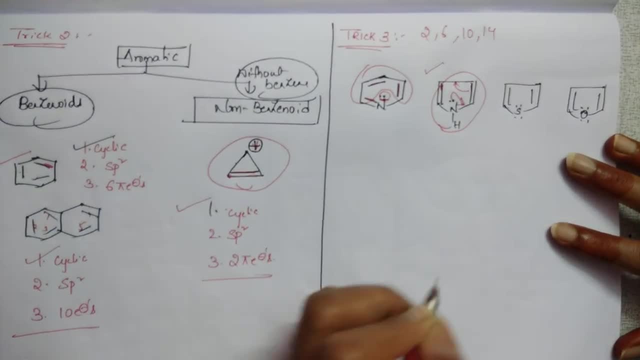 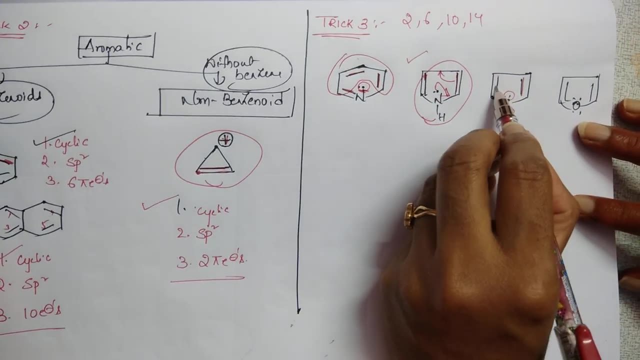 involves in a resonance total 6 electrons. it is also aromatic, see in this case 2 plus 2, 4. now here 2, here 2. is there total? how many? 2 plus 2, 4? and here 4 plus 2, 6 is plus 2, 8. total 8 is. there 8.. it is anti-aromatic. if you consider your answer is a wrong answer. why it is a wrong answer? because this 2 electrons involves in a resonance. in this case, with this 2, it is becoming 6. once it is becoming 6 it- these electrons- don't involve in a resonance. it is ready to donate? ok, see in this. 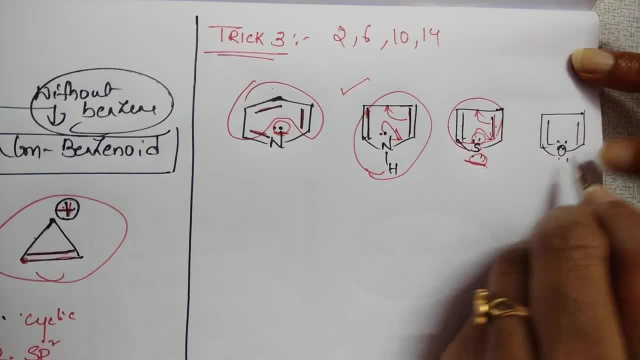 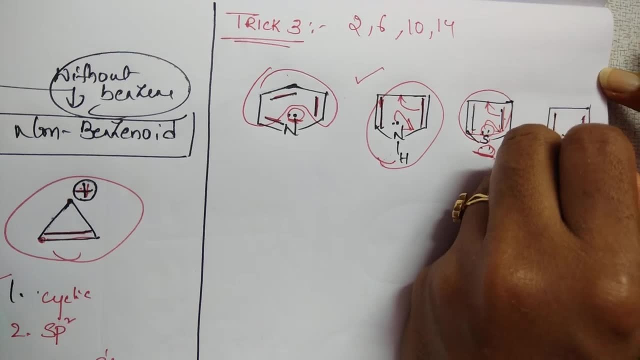 case furane. what happens? here total there are 2 lone pairs, so in this 2 lone pairs is 2 lone pairs will involve no, here 2, here 2, total 4 and here 2, 6. so with this 6 only it is getting aromaticity and this 2. 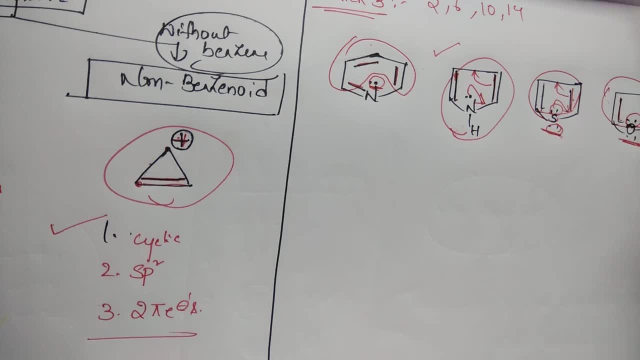 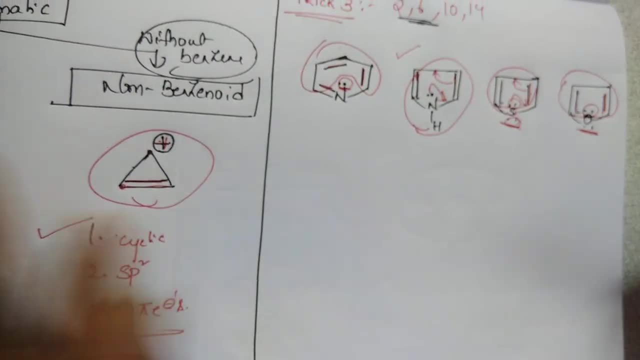 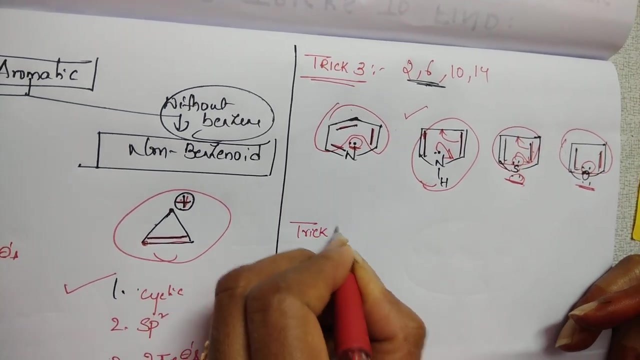 electrons dont involve. so in such a way you have to calculate, simply total, you count and you will get the wrong answer. you should check if it is already getting aromaticity with 1 lone pair means then you don't need to count the other lone pair. trick number 4: here I want to discuss about 2 types. 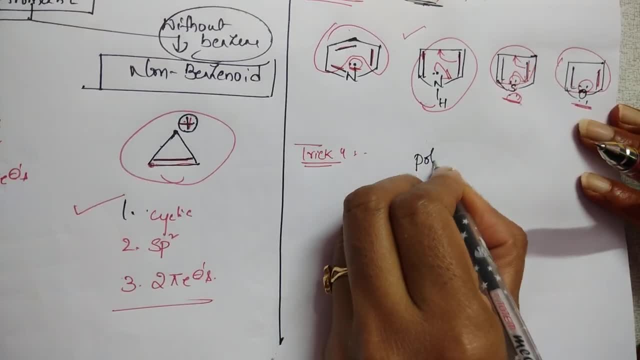 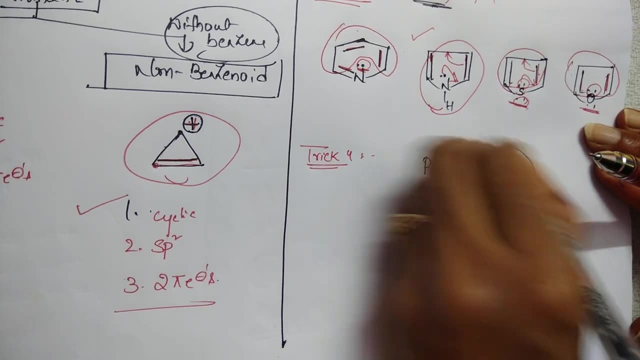 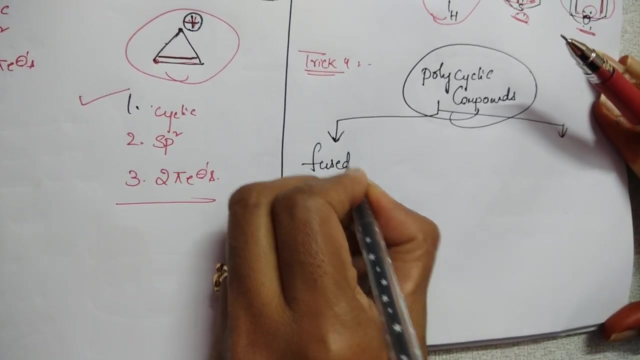 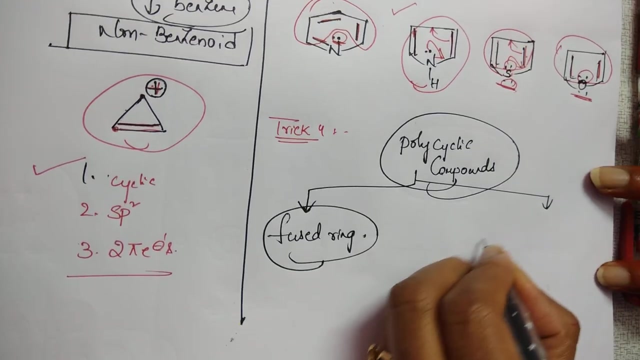 of aromatic rings. ok, ok, ok, ok, we call it as polycyclic compounds. What are these polycyclic compounds? These polycyclic compounds are of two types. One is fused ring containing compounds. What are these compounds? students tell me Fused ring containing compounds and another one is another one, is you know? 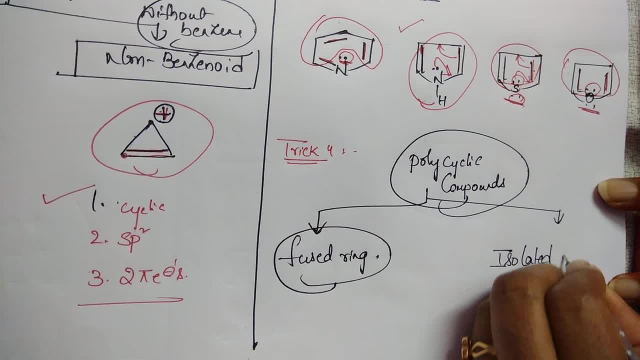 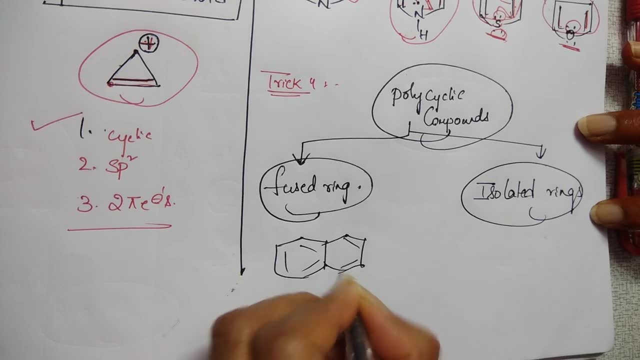 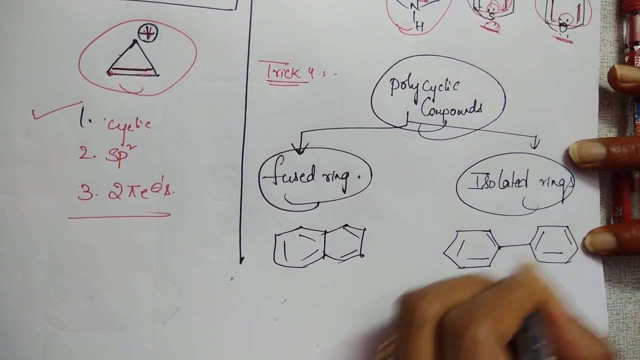 isolated rings, Isolated rings. What do you mean by fused rings? If the two rings are connected like this, then it is a fused. If suppose the two rings are separated by a single bond, like this, or a one bond is there, then it is called as isolated In fused rings. what you have to do? 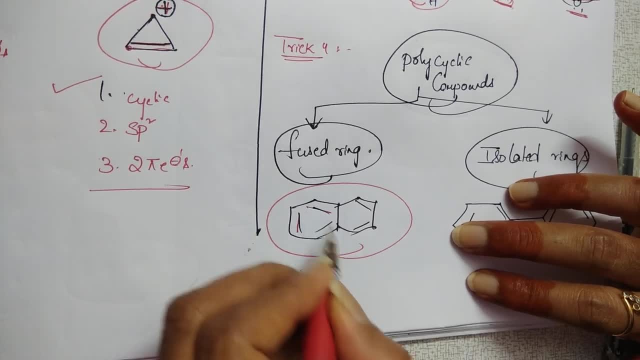 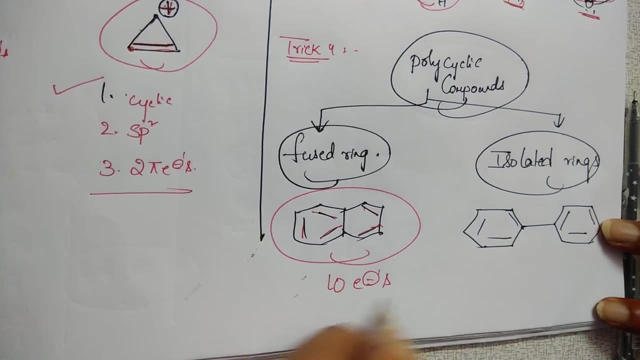 is you should count the total number of electrons: 2 plus 2, 4, 4 plus 1 bond contains 2 electrons, total 5 bonds. So 5: 2's are 10 electrons. So 10 pi electrons means aromatic See here. Here 3 bonds. 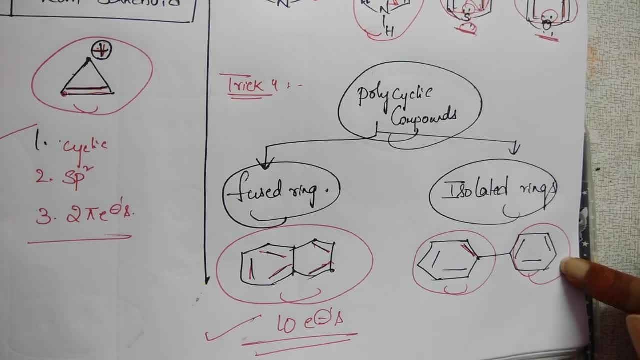 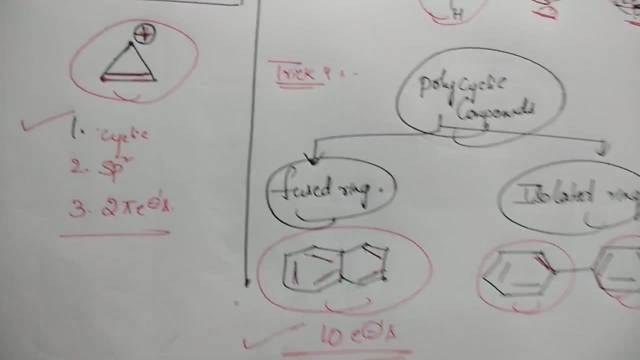 3: 2's are 6.. Here, 3 bonds 3: 2's are 6.. 6 plus 6: 12.. If you consider 12, then it is not aromatic. Okay, Then your answer is a wrong answer. So what do you have to do? Clear no. What do you have to? 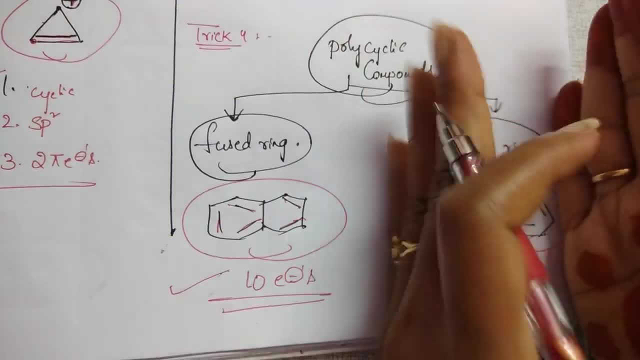 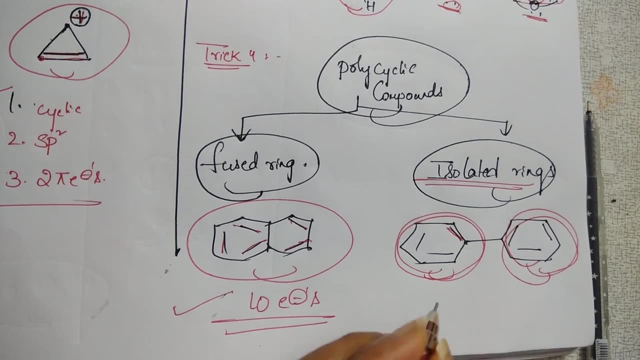 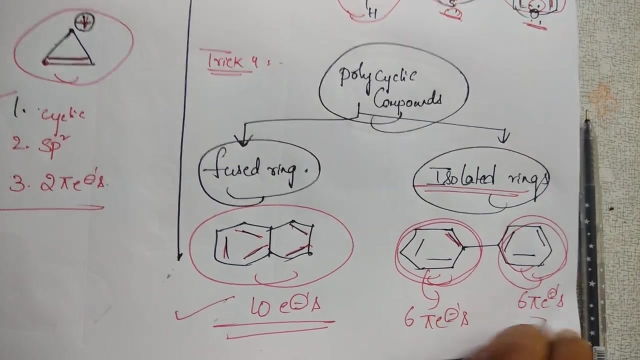 do? You should not consider this together. This is an isolated rings. This ring separated, you should count, and this ring separately, you should count. So this ring have 6 pi electrons aromatic and this ring has 6 pi electrons aromatic. So in such a way you have to do. 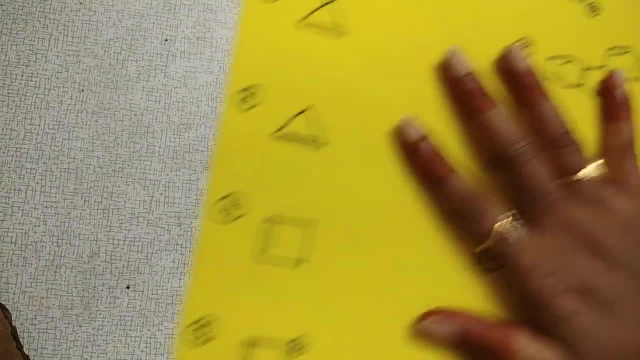 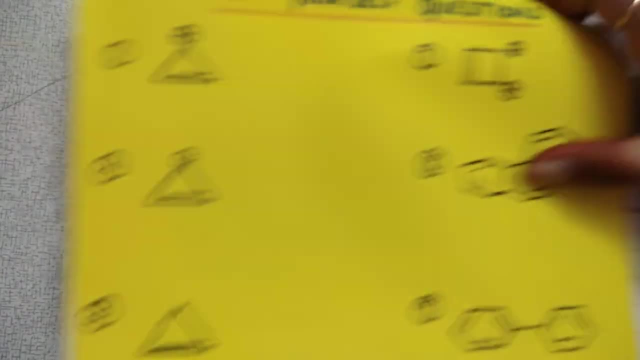 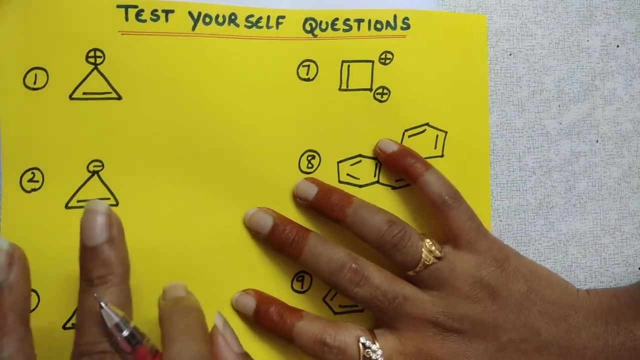 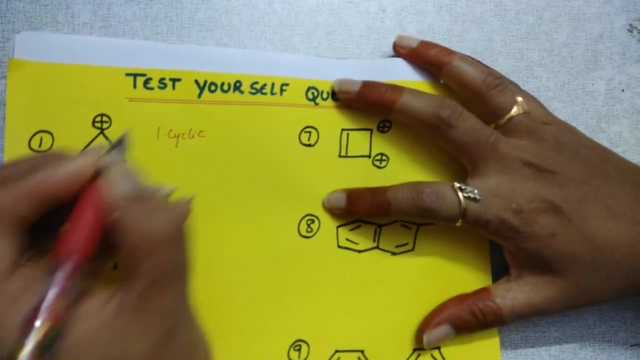 Let's begin the question solving. Try these questions. Come on everybody. Question number 1.. First thing: it is cyclic or not. can you tell me Question number 1.. See the first question. how easily we will do. you know, You see a lots of difference. It is cyclic. First condition is satisfied, Must condition. 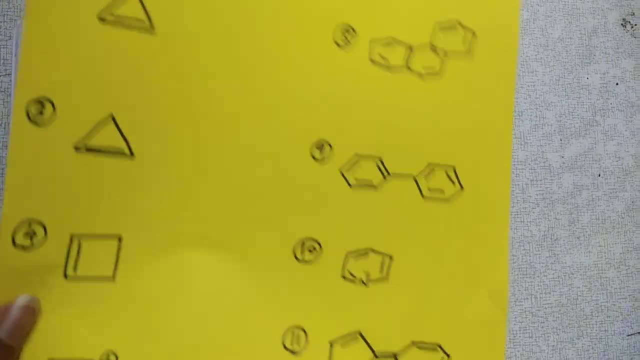 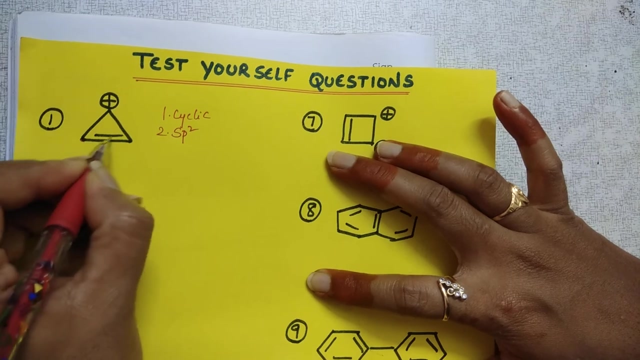 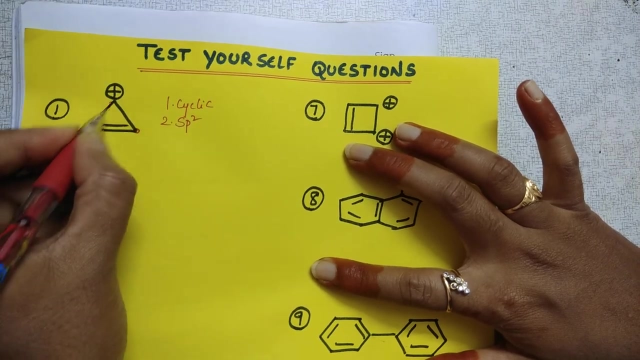 it should be cyclic. So every of this structure is cyclic, So I am not going to write it, Okay, Again and again. Second one is: every carbon should be sp2.. So this is having a double bond, so sp2.. This is also having double bond, sp2.. Then how to find this one? Pi sigma single. 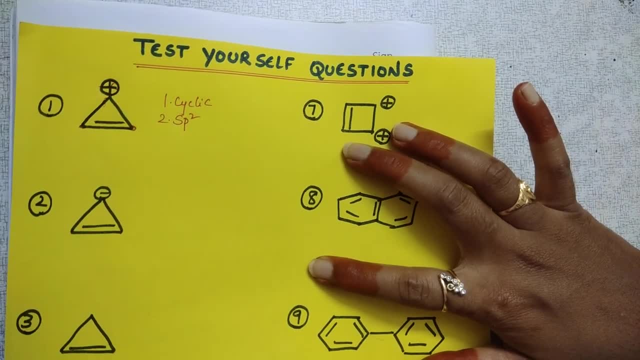 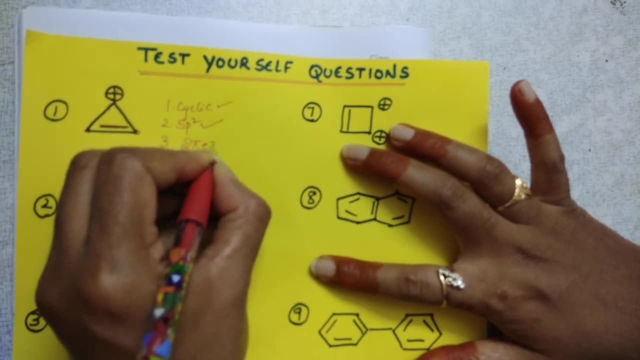 bond Positive charge. So pi sigma positive charge is there, It is sp2.. Okay, This condition also satisfied. Third, one Total number of pi electrons are 2.. One bond contains 2 pi electrons. So this is what condition. students tell me It is aromatic. 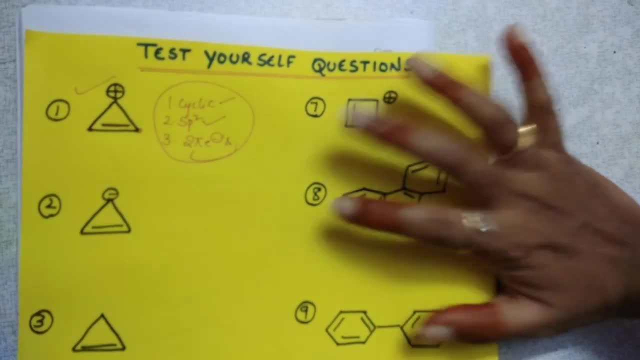 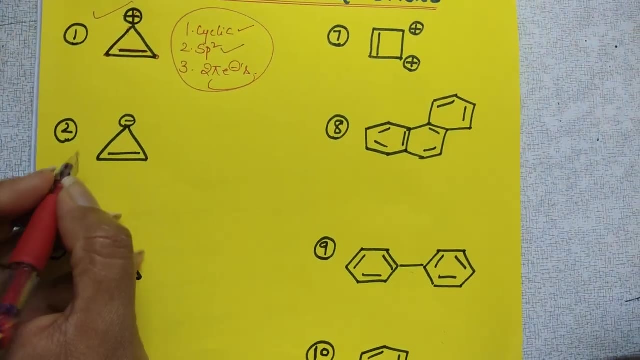 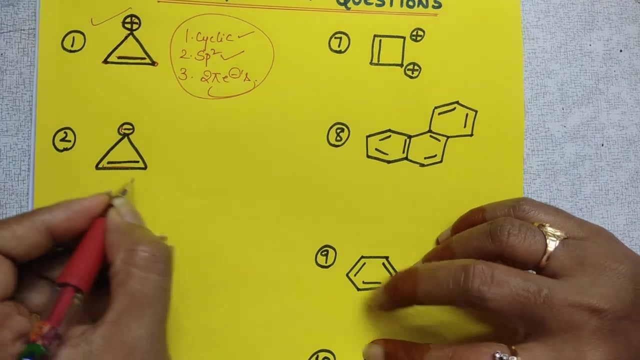 Is it clear? Is it clear? Now try the remaining also. See the second question. It is cyclic and the second condition is it is sp2 because pi sigma positive charge is there. So it is sp2 and total number of pi electrons. 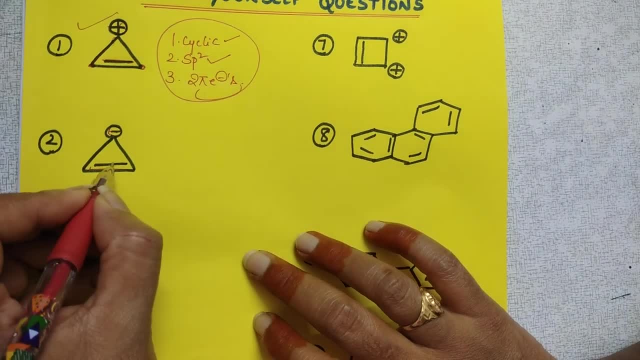 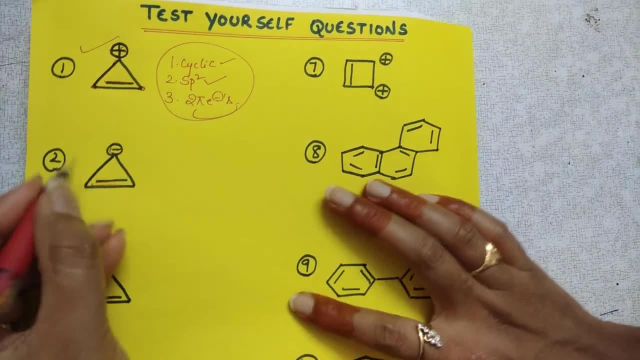 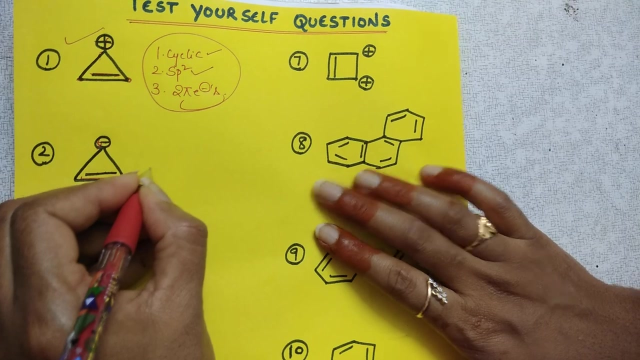 How many In this case Can you count and tell me: Pi sigma positive charge is there? Come on, Yes, Very good. So here 2 electrons and these 2 electrons also involves in the resonance Pi sigma negative charge. total: 4 pi electrons are there. Then it is following: 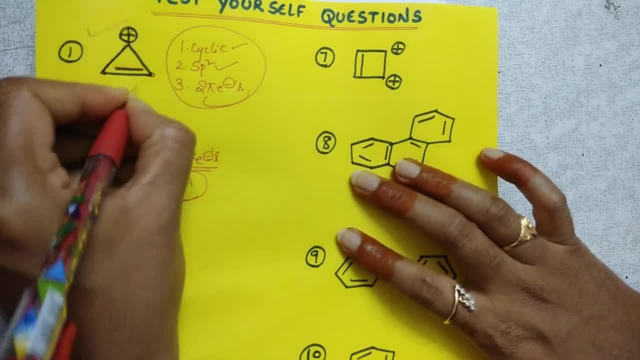 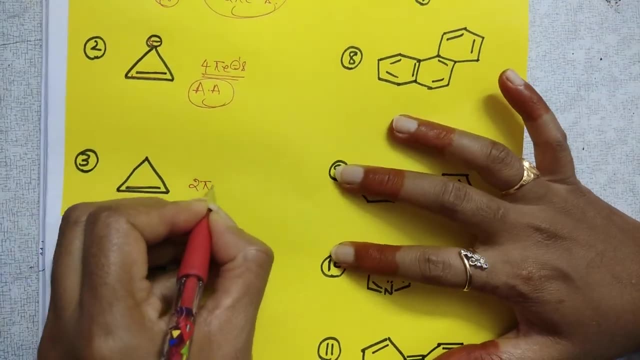 anti-aromaticity, This is anti-aromatic, This is aromatic. See the next one Here. pi bond is there, Cyclic is there. Two pi electrons are there, Fine, And it is cyclic, Fine. But here this carbon is having. 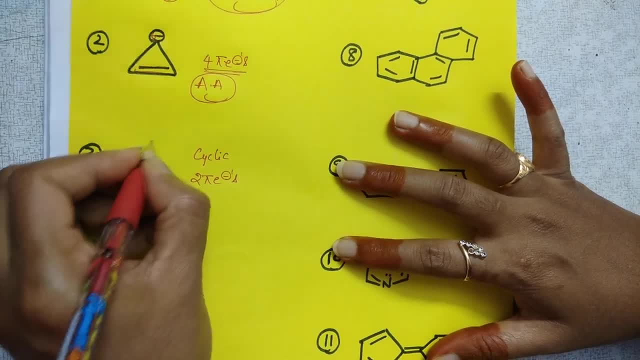 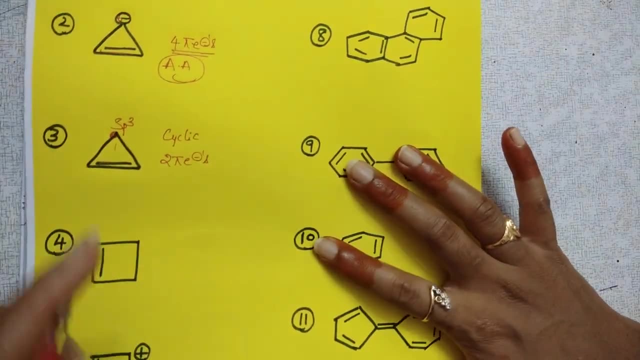 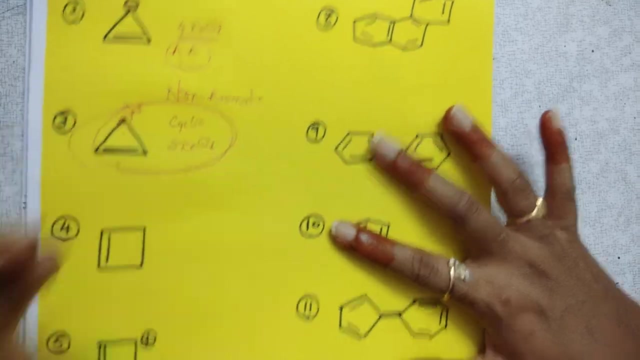 only single bond, this side and this side, which means that this hybridization is sp3.. If any one of the condition, if it is not following, then it is which structure? can you tell me? students, It is anti-non-aromatic. It is non-aromatic, See the next one. Can you tell? 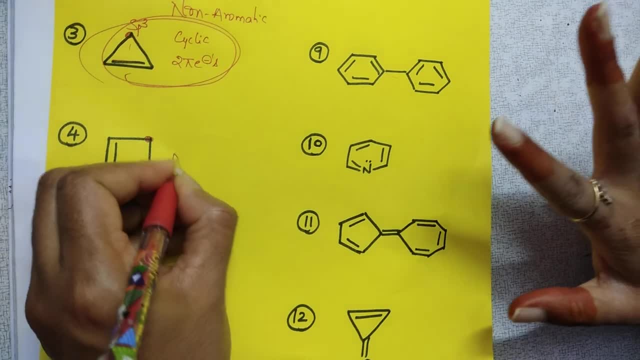 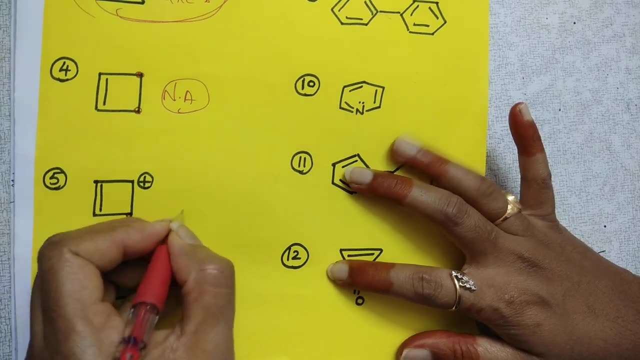 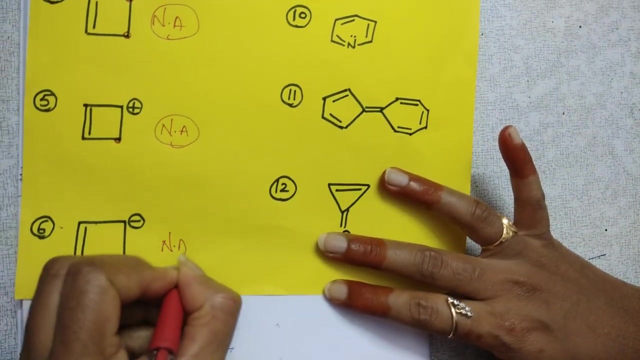 me the next one here: Sp3 hybridization is there itself. It is non-aromatic. It is non-aromatic. Then see the next one: here, Single bond is there, Only single carbon is there. Then it is non-aromatic. And see here: Single carbon is there, Non-aromatic Means, it is cyclic. 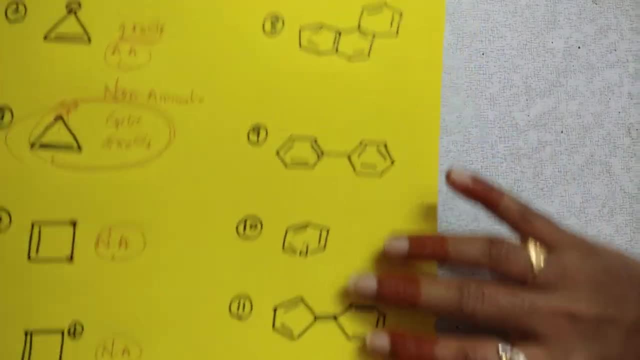 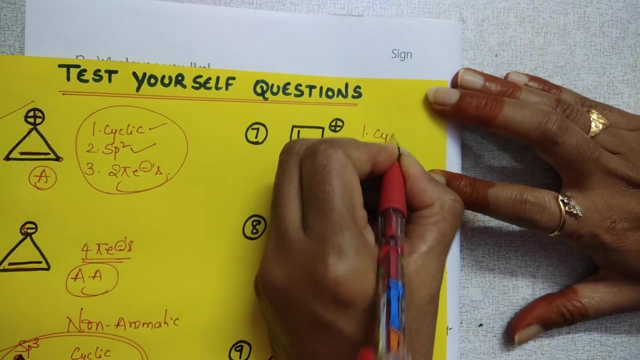 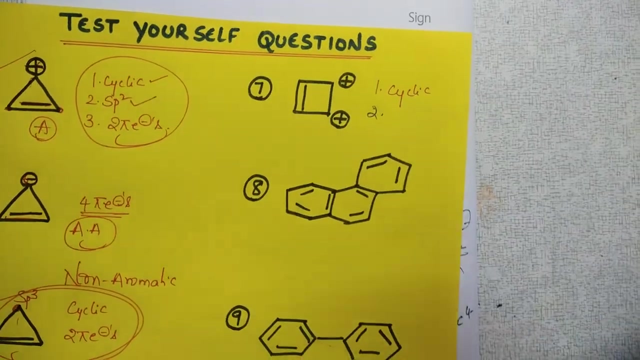 It is showing resonance, But it is. you know, sp3 hybridization is there, means it is non-aromatic. See, in this case. now, First one is it is cyclic. And let's see the second condition. Is it clear? Is it clear? Second condition: you see, This structure is sp2 hybridized. Very good, And 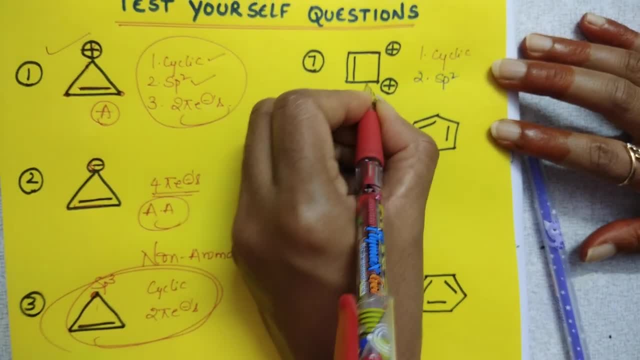 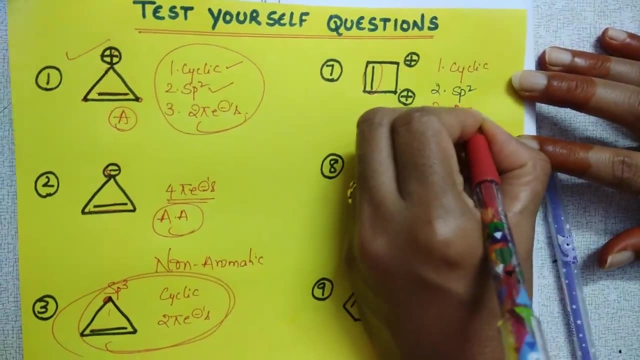 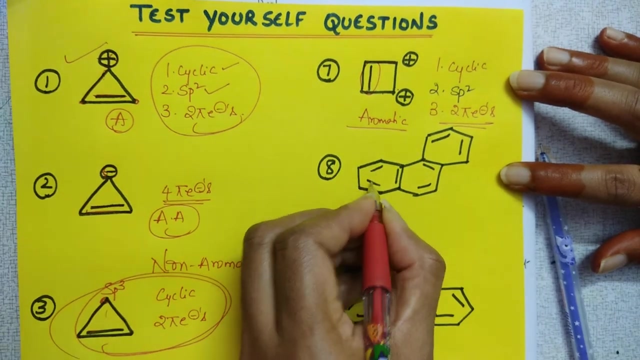 the every carbon, because pi sigma positive, Pi sigma positive, sp2.. And the third one is it is having total 2 pi electrons. 2 pi electrons, So it is aromatic. Then this structure is aromatic, See the next one: 1,, 2,, 3,, 4,, 5, 6, 7.. 7, twos are 14 pi electrons Every carbon. 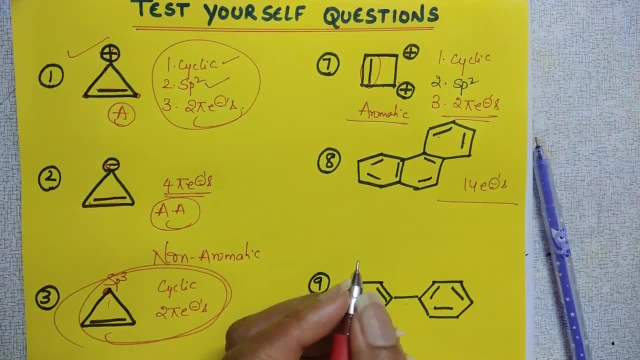 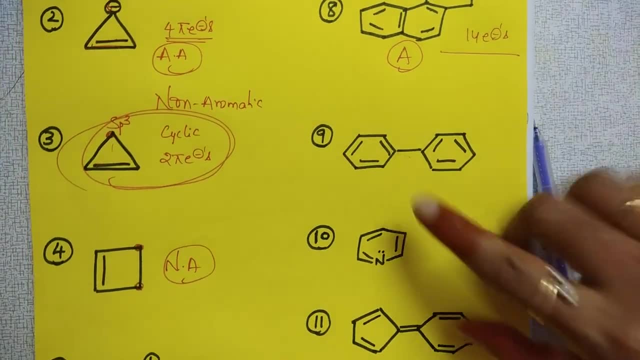 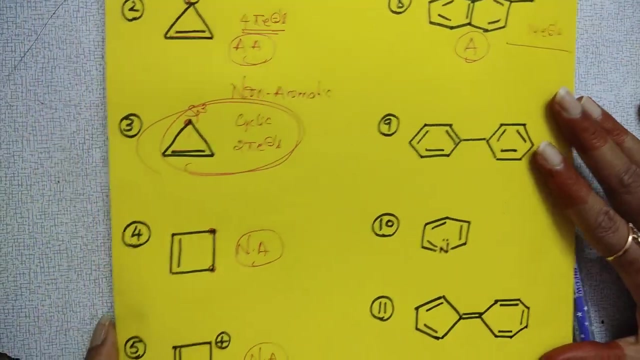 sp2.. Every carbon, you know total structure is cyclic, So 14 pi electrons are there. So it is also aromatic. See. in this case It comes here: 3 pi bonds, 3 twos are 6. here, 3 pi bonds, 3 twos are 6.. 6 plus 6 is 12. if you do, Then your answer will be the wrong. 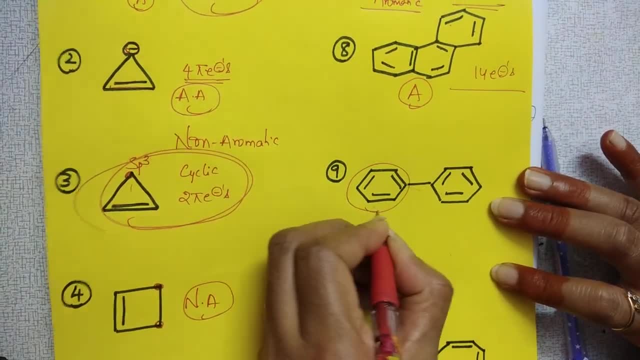 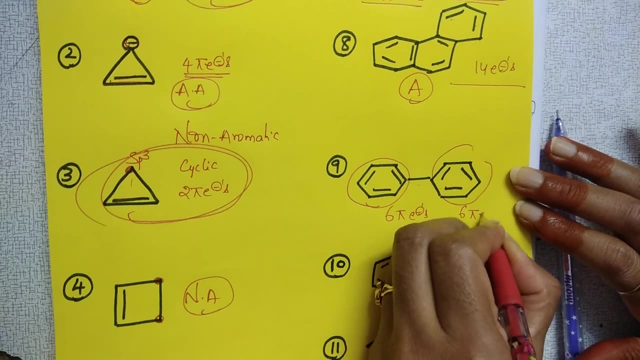 answer. Why wrong answer? This is a isolated ring. This separately, you should count This separately. you should count. Then it is 6 pi electrons in this case And 6 pi electrons in this case. So this is the isolated ring. This separately, you should count This separately, you should. 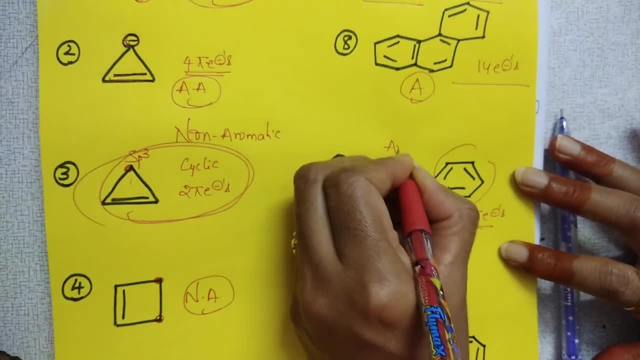 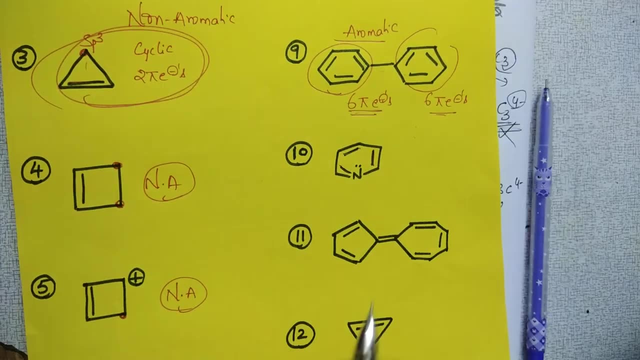 see the following: Students, is this clear? So this is also aromatic. Aromatic. Now see in this case 1,, 2, 3.. 3, twos are 6. And if this also involves, it becomes 8.. No, It is. 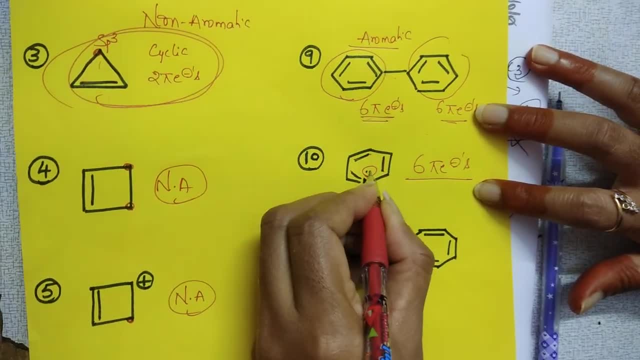 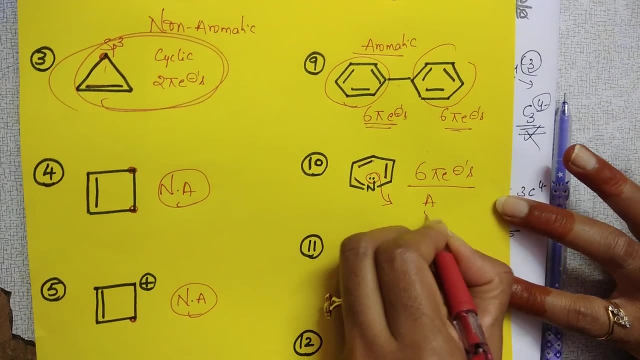 enough 6 pi electrons you should consider. But this lone pair you know it is free to donate, It acts as a good base. Pyridine likes to donate, So it is aromatic And we should not count this lone pair And see the next case. 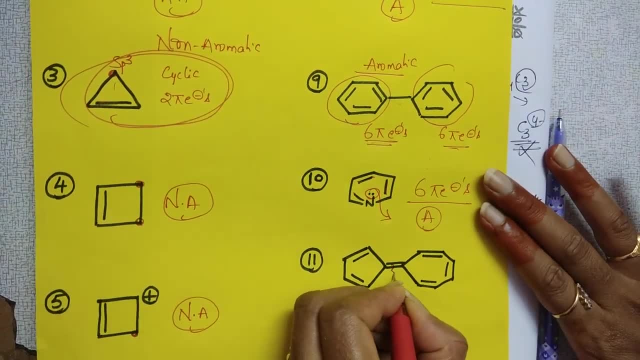 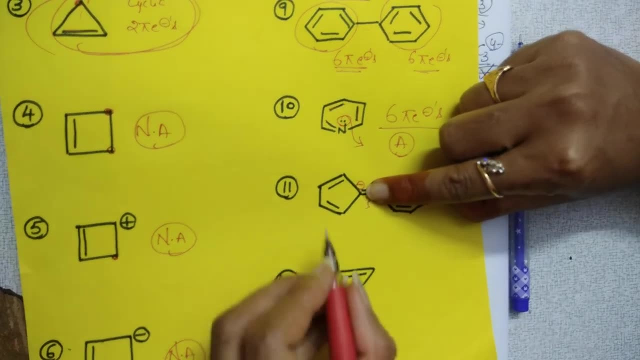 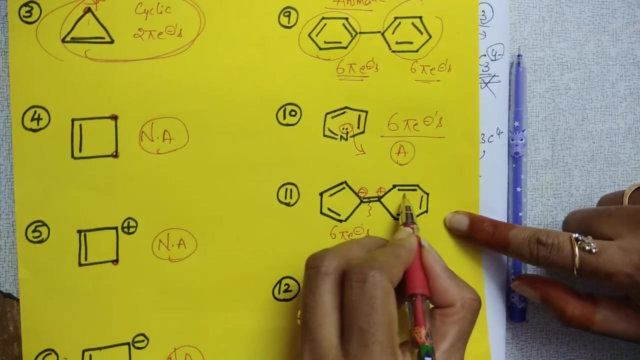 Where there is a rigid double bond is there, Then you try to break this double bond. One side you keep positive charge, Other side you keep negative charge. Then if you count 2 plus 2 plus 2.. Total 6 pi electrons it is getting This side you count 2 plus 2 plus. 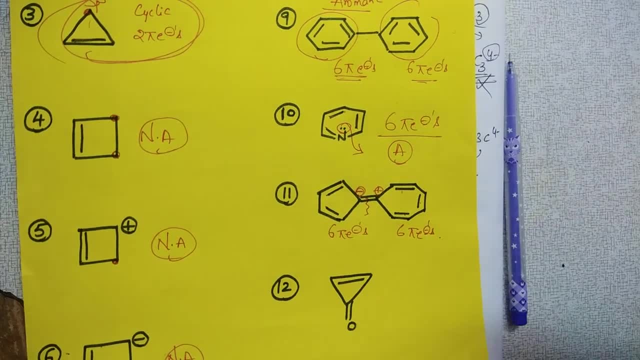 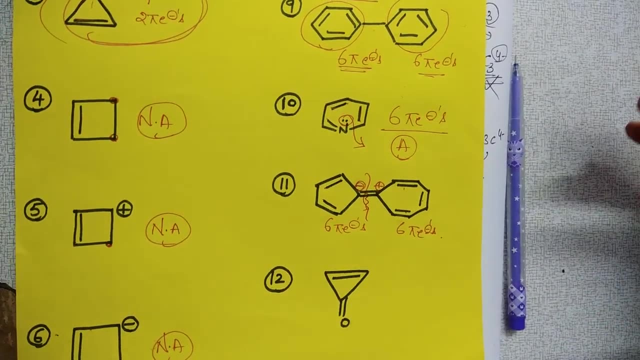 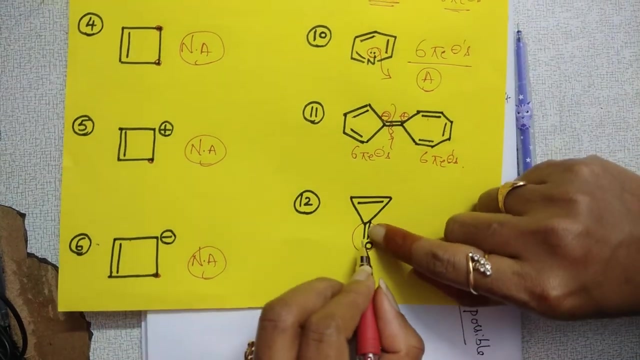 2. 6 pi electrons. So this ring likes to break and it likes to involve. you know, this type of This like to break like this, Not in a reverse direction, See the next question. This is the out of the ring. So within the ring only pi bond.